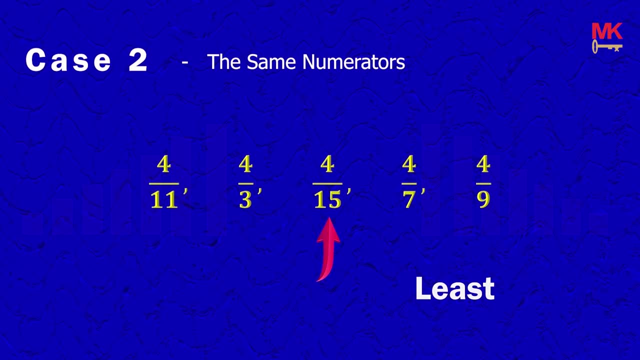 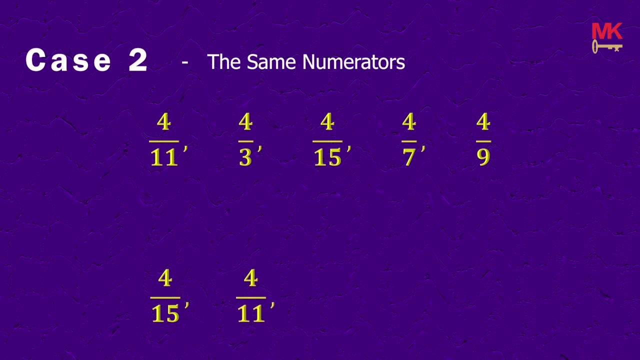 among these fractions, the least in value is 4 over 15.. Arranging them in ascending order, the next becomes 4 over 11, followed by 4 over 9, 4 over 7, then 4 over 3.. While in descending, 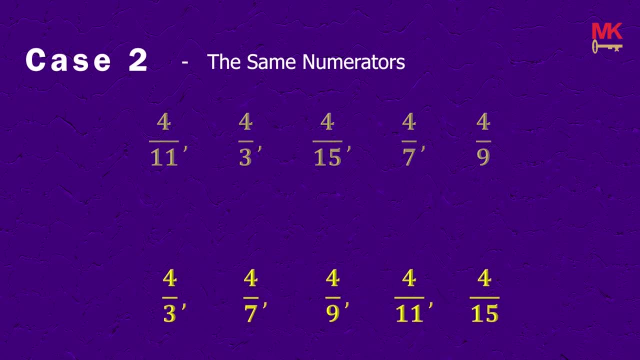 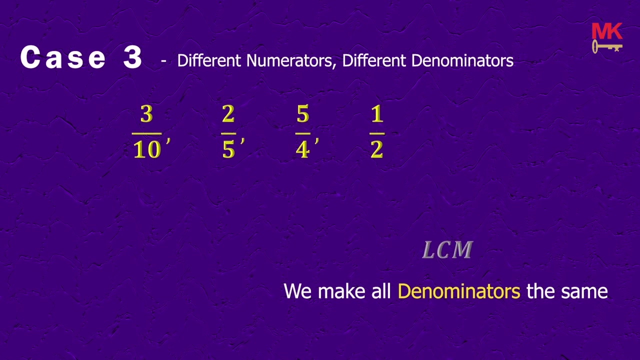 order. we just reverse the order of arrangement without stress. In this case, all numerators are different, all denominators are different. So what do we do? Excellent, We make all denominators the same by finding their LCM. From our multiplication table, the LCM of the denominators is 20.. In other words, we are going. 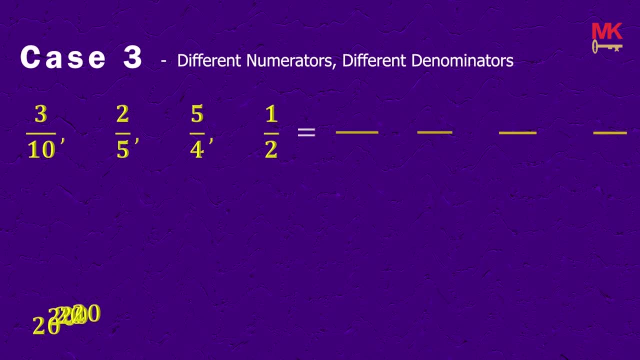 to rewrite the fractions in such a way that they all have common denominators. Now that all denominators have changed, we will also need to get the corresponding numerators and then we compare the fractions by their numerators, just as we did in the previous example. But the question 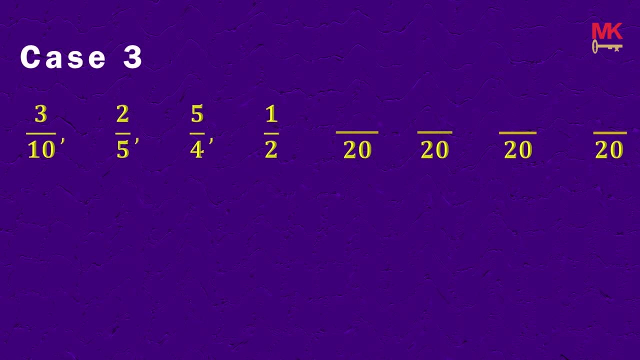 is how do we get the numerator for each of them? Well, that's a whole lot easy to do. For the first fraction, its denominator goes into the LCM, and that's exactly 2.. Then we multiply by its numerator. Everything on top becomes 6.. For the 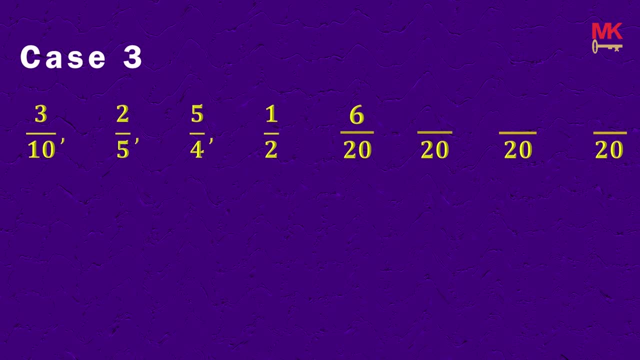 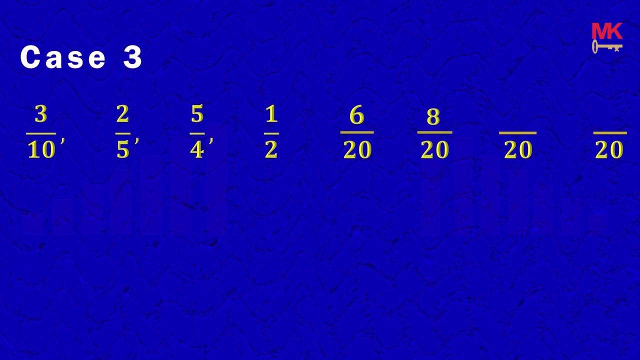 second, we repeat the same process. Its denominator 5 goes straight into the LCM, which gives 4.. Then we multiply by its numerator, So everything on top becomes 8.. And we repeat the same process. The third fraction becomes 25 over 20 and the fourth becomes 10 over 20.. 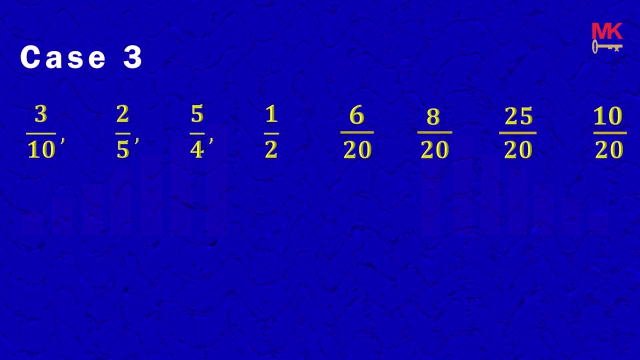 Amazing. This is really getting interesting. The fractions now look like those in case 1, being that they all have the same denominators. Comparing them, the greatest in value becomes 5 over 4.. And the least in value becomes 3 over 10.. Note that, by virtue of all theز.